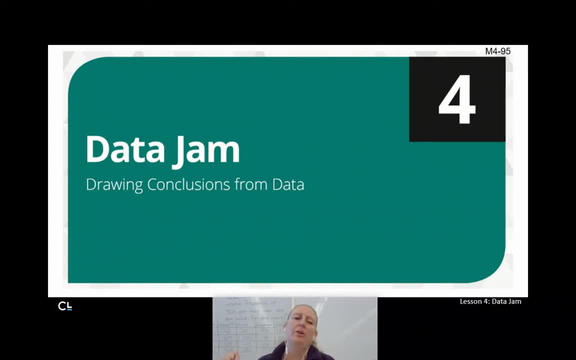 Hi, integrated math one. Welcome to lesson two. point- pardon me, I'm going to try this again- 4.2.4b. Yes, that's where we are. We're on day two of drawing conclusions from data. So we've been making all kinds of tables, all kinds of graphs, and now we're just trying to draw conclusions from it. right, What patterns do we see? What decisions can we make based on what we see? right, That's all we're looking at these days. So that's the big thing about data: making decisions from it. So remember, Andres. 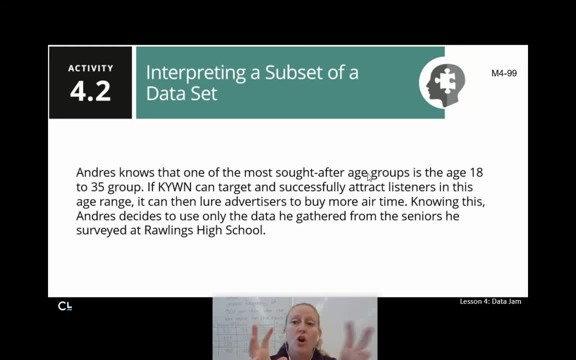 on page. we're now on page M4-99.. If you recall, we made a table with Andres's data. we made a graph- right, a stacked bar graph- with Andres's data And they were trying to make some decisions about the radio station that he's now the manager of and whether we should change it or not. So we decided to do a survey at Rawlings High School. he decided to, you know, host the dance and the data was was nice but felt like it was kind of close to numbers and things could shift a little bit. 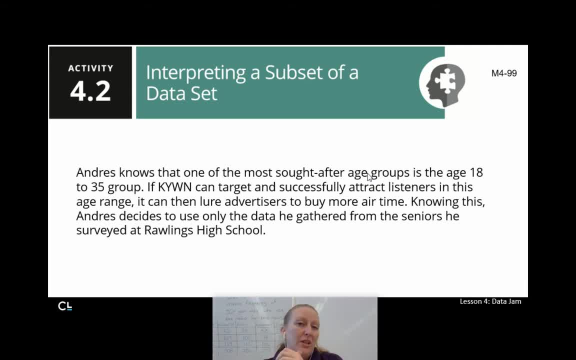 So Andres knows that one of the most sought after age groups in the radio business is the age 18 to 35 group. If KYWN can target and successfully attract listeners in this age range, it can then lure advertisers to buy more airtime. That's how the radio station makes their money right. So, knowing this, Andres decides to use only the data he gathered from the seniors right. 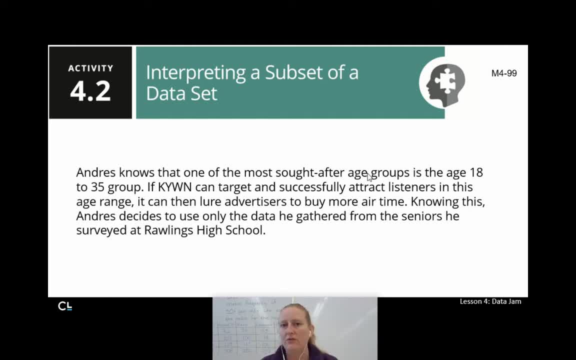 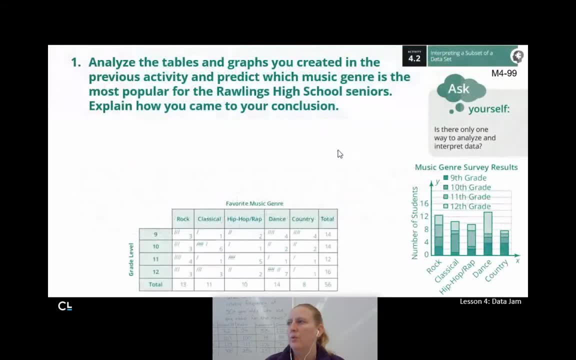 So we're going to analyze the tables and graphs that we created last time And we're going to predict which music genre is the most popular for the Rawlings High School seniors. So go ahead and write down which music genre do you see is most popular for the seniors and tell me how you came to that conclusion. Hit pause. write it down. 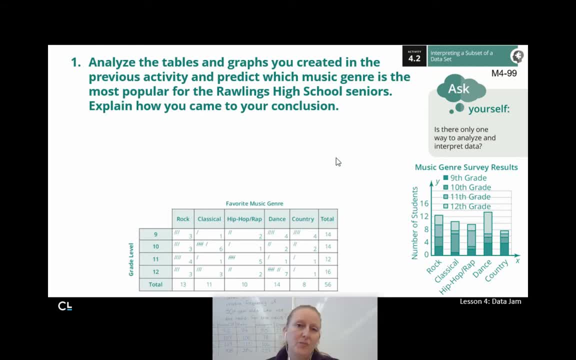 Hit play when you're ready to check your work. So we're only looking at the seniors. So on this graph, this means I'm only looking at those top chunks of my stacked bars. Or, of course, if you're looking at the table, in this case I find a little easier to use the table. I'm just looking for the biggest number here and I can see it's in dance, And even as I look at the stacked bar graphs I can see that. that 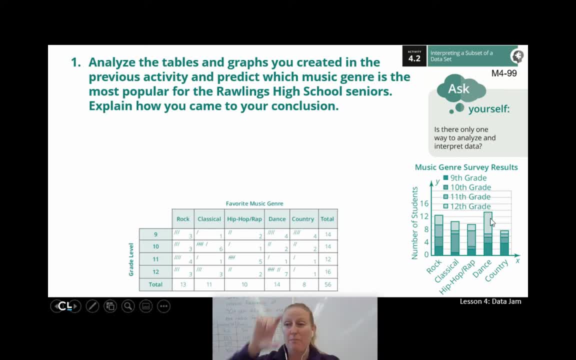 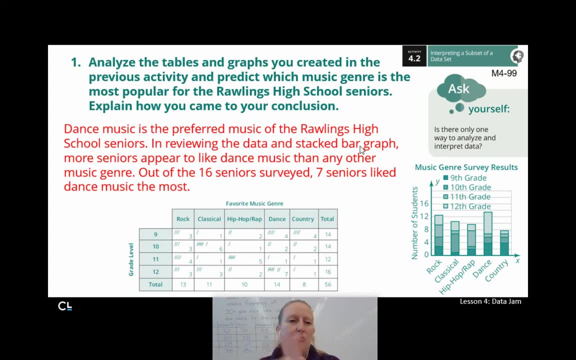 in the. it's in the dance section that the seniors have the biggest bar. So I'm going to say dance music is the preferred music of the Rawlings High School seniors. Whether I'm looking at the data in the table or the stacked bar graph, more seniors appear to like dance music than any other music genre Like. out of the 16 seniors surveyed, 7 seniors liked dance music the most. 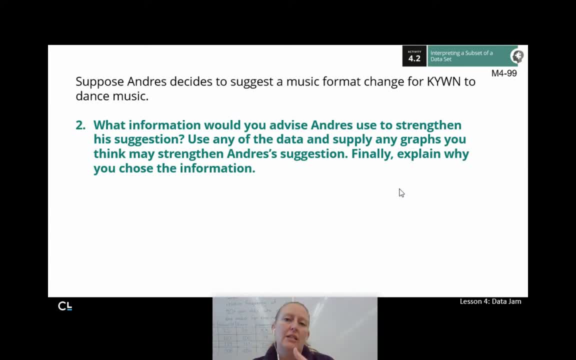 So suppose Andres decides to suggest a music format change for KYWN to dance music, dance music. What information would you advise Andres use to strengthen his suggestion? And you can use any of the data, supply any graphs you think might strengthen his suggestion and explain why you chose the information. So go ahead, hit pause, jot down your thoughts. 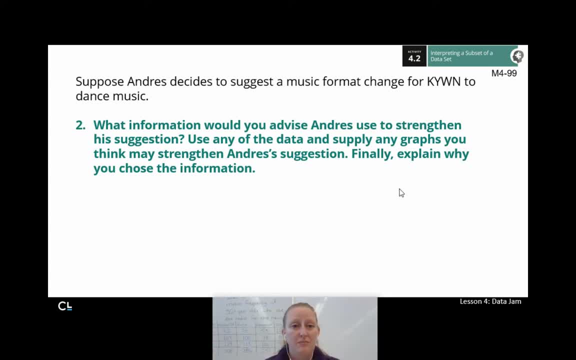 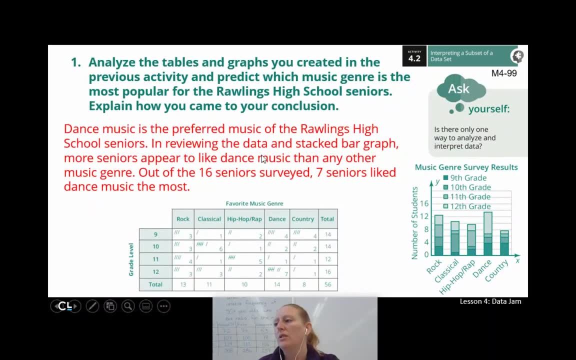 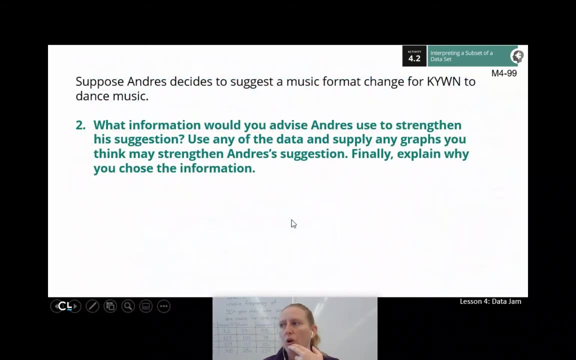 hit play when you're ready to check your work. So my thought on this is, instead of using the whole table, I just want to focus in on those seniors, on those 12th graders. So my thought is, instead of the whole table, let's use a conditional relative frequency. 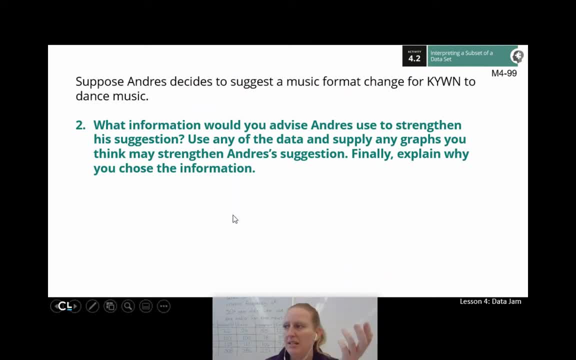 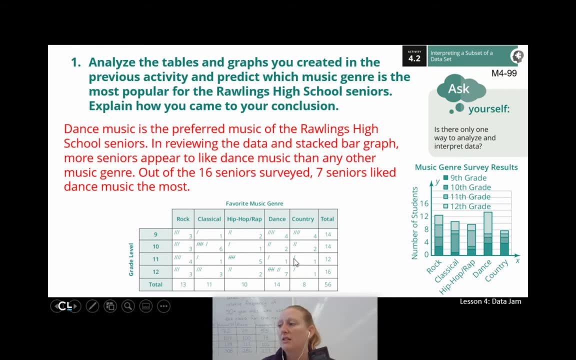 graph table right. Instead of basing it out of everybody, let's come back here and do all of these numbers out of 16 and do my percent. So 3 out of 16,, 3 out of 16,, 2 out of 16,. 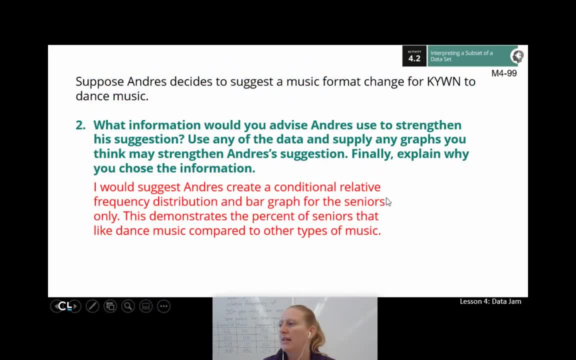 7 out of 16,, 1 out of 16.. And I'm going to turn those into percents And this gives me a nice direct comparison. that also means if I wanted to do a graph, I could do a graph with percents, right, And then I would just have one bar for each one And I'd be like: 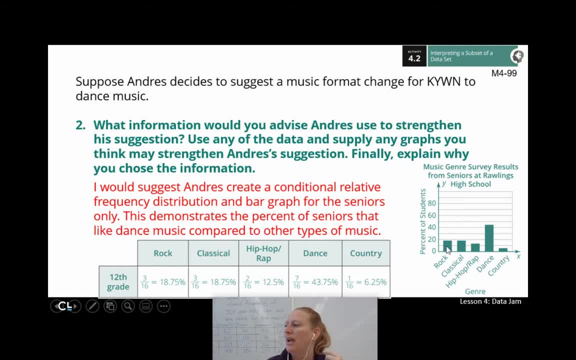 my rock bar, my classical bar, my hip hop bar, my dance bar, my country bar, And now I just have my seniors. So if Andres is like we need to change the music format to dance and he wants to prove it with numbers, he can use the conditional relative frequencies. 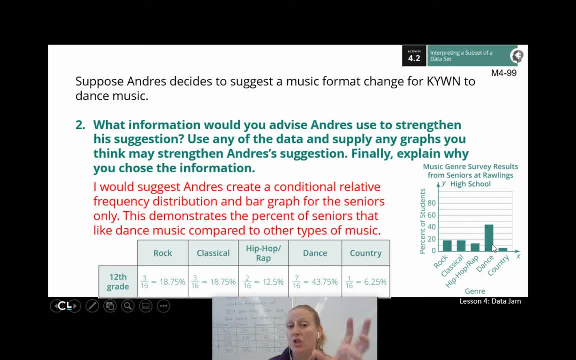 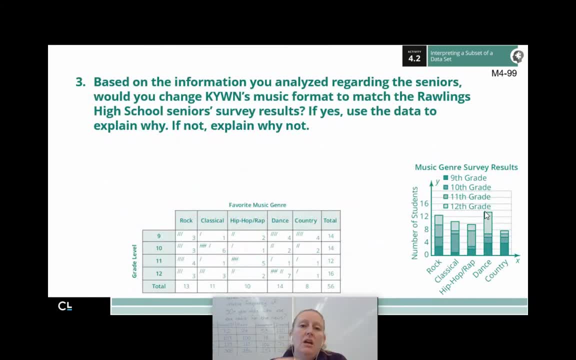 just comparing 12th graders to 12th graders. He can use a graph with just the 12th graders on it to help strengthen his argument. Now, based on the information we analyzed regarding the seniors, would you change KYWN's music? 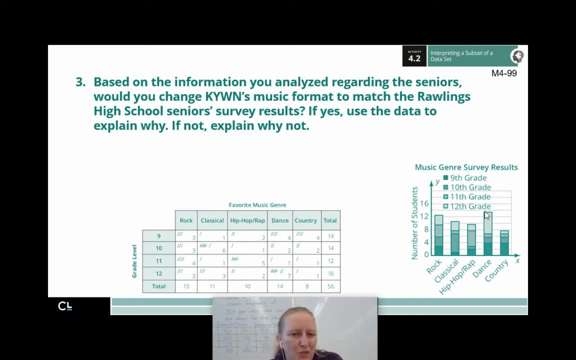 format to match the Rawlings High School's seniors survey results. If yes, use the data to explain why. If not, explain, why not Hit pause? Jot down your thoughts, Hit play when you're ready to check your work. So here's the thing I mean. the seniors are 18, 19 years old, and I get it. so that's. 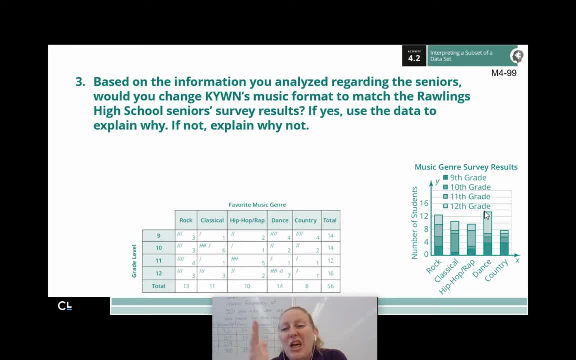 good data, But remember the demographic was 18 to 35-year-olds. I feel like if I'm only using data from 18 and 19-year-olds, that's not enough to advise that big of a change, Because the target age group is bigger than that. I really think Andres should conduct. 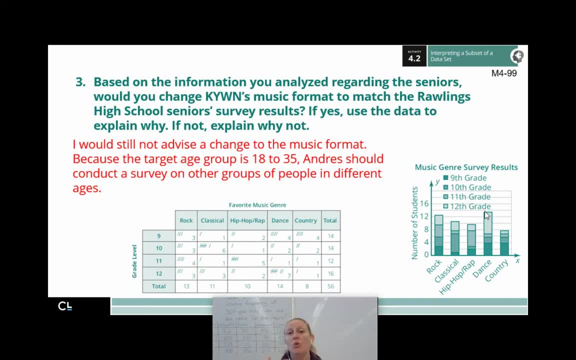 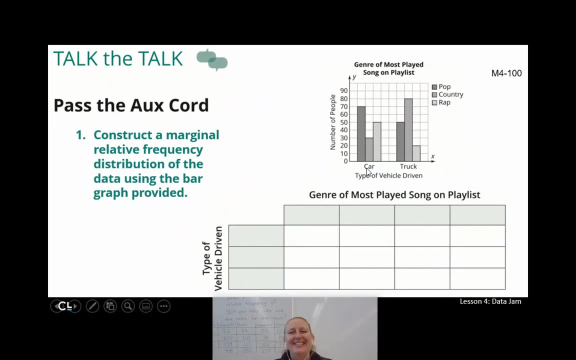 a survey on other groups of people in different ages. right, He needs to conduct some surveys that get in all of those age ranges, all the way up to 35, instead of just a bunch of high school seniors. That's just my feelings on the subject. 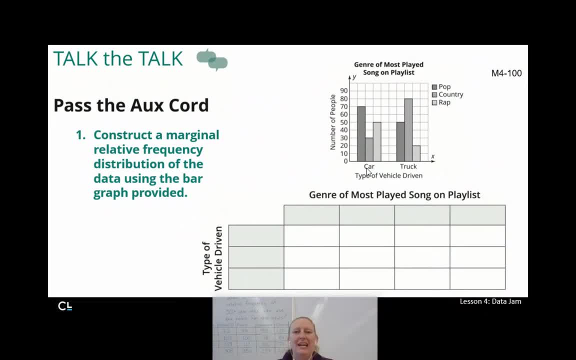 Let's do just a little bit more on page M4-100.. This is interesting. In the past we've been conducting, we've been creating our tables and then using our tables to make graphs. I want you to go the other way around. 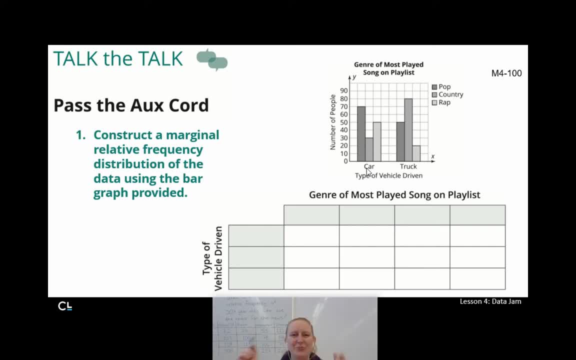 Use your graph to make the table. What Can you do it? Can you go backwards? Please notice, it's a marginal, relative frequency. Oh, oh oh. That means I want you know how this goes. this means that I want percent people. So hit pause, Hit pause, See if you can fill. 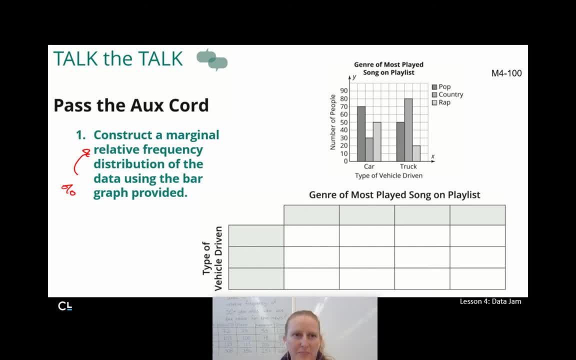 in this table. Hit play when you're ready to check your work. So first of all I need to like, fill in all the boxes here. It looks like type of vehicle driven. I have a car or a truck. Put that on there. Yay, car or truck. And it looks. 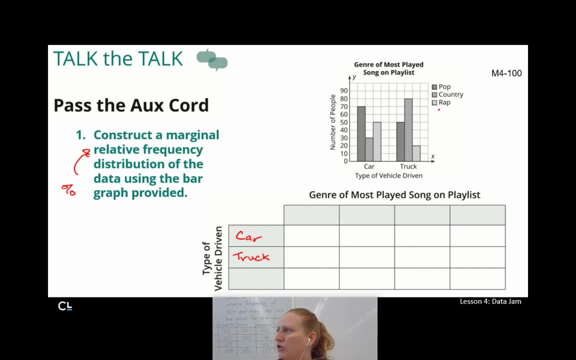 like I have three different kinds of music right. I've got pop, country and rap, So I'm going to put that pop, country and rap, And then, of course, I'm going to put my totals over here. Let's start. I'm going to fill in the straight numbers and I'm going to put them kind of. 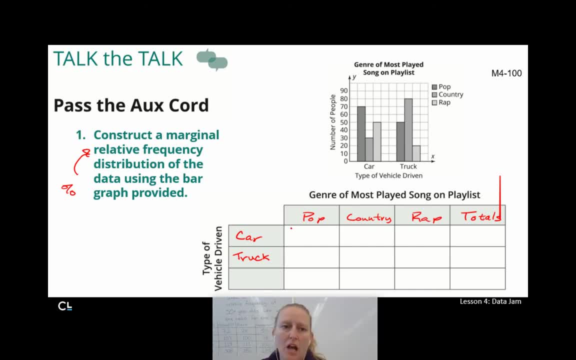 in the upper corner over here. I'm just going to put in the straight numbers that I have And then I'll stress out right, And then I'll worry about the rest of this. So it looks like car pop in the car is 70. Country in the car is at 30. And rap in the car is at. 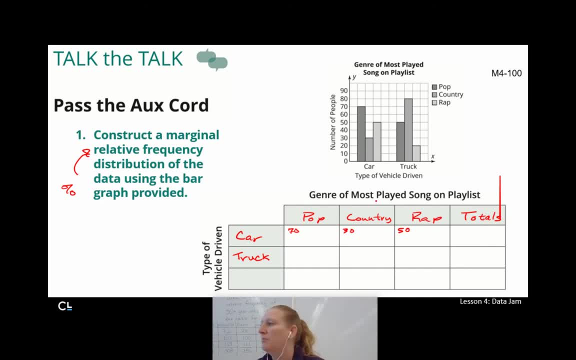 50. Like I said, I'm going to do stuff with these numbers. That's why I'm making them so small. Let's see What do I have here. Pardon me, Pop in the truck is at 50. Country in the truck is at 80. Okay, apparently, if you drive. 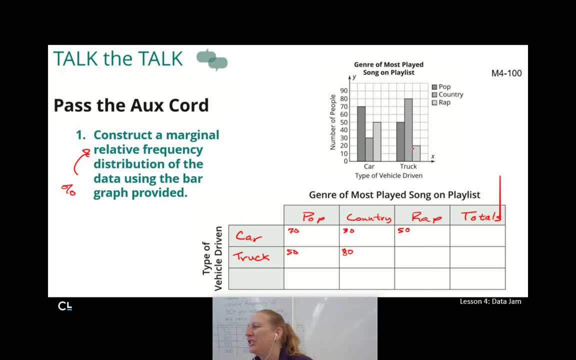 truck. you really like country music And rap in the truck is at 20.. I do want to get my totals in here if we're doing marginal stuff, So I am going to grab my calculator real quick and add some things up. If I do 70 plus 30, that's 100 plus 50 means I'm at. 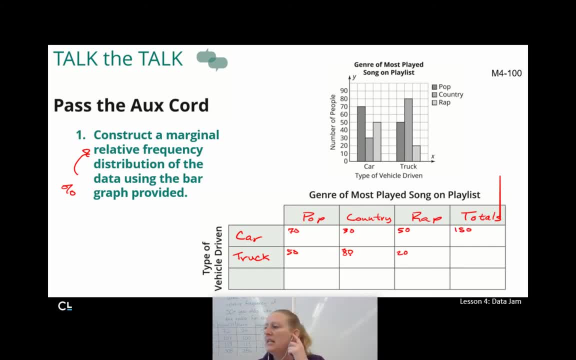 150.. 50 plus 100.. Okay, 80 is 130 plus 20.. Oh, also 150.. Okay, cool, Great. Which means, if I add these together, my total total is 300.. If I add these together, I'm at 120.. If I add those together, I'm at. 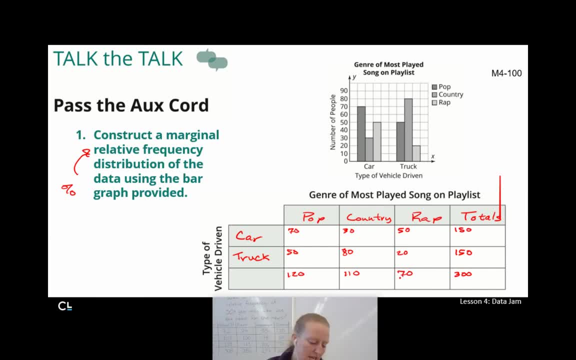 110.. And if I add these together I'm at 70.. Now it did say the marginal relative frequency, So I'm going to divide everybody by 300.. Literally all of them, All of these are going to be at a 300. 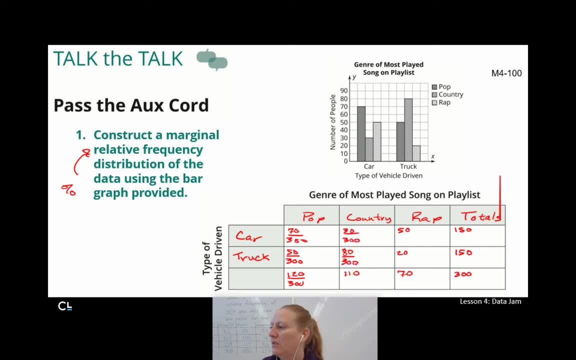 And this is why I love my calculator, because, oh dear. So all of these are going to be at 100.. We're going to divide out of a hundredPardon me, All these are going to be out of 300. Since I do want a percent, we're going to divide all of these by 300 and then multiply by 100 in order to get a percent. So I'm going to grab my calculator here, And I've already done that, And what have I got? 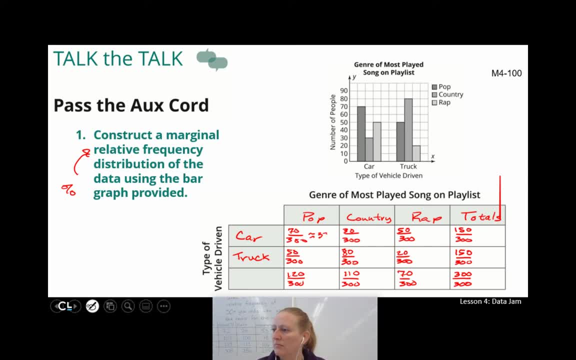 here, I've got about 23.. Oh, dear Miss Scala, And what I've got here? We have about 25.. Okay, Ms Scott. Ms Scott, I am using a wavy equal sign because it is approximately so 23.3%. 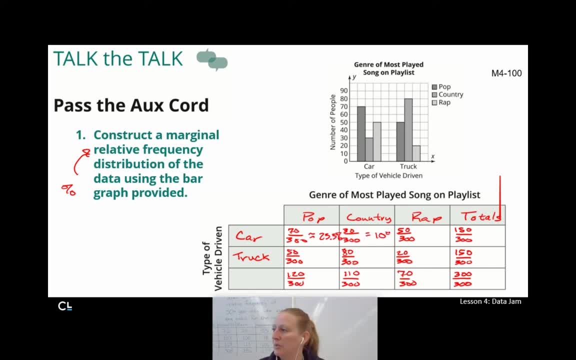 That one's exactly 10% as convenient. This one is about 16.7% And of course, this is exactly 50%, which means that one's also 50%. I'm going to come down here. So 50 out of 300.. I think we. 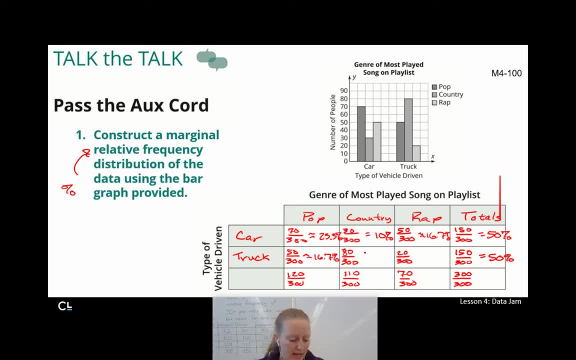 did that one earlier at 16.7%. 80 out of 300 is about 26.7%. 20 out of 300 is about- oh, that's small, It's only about 6.7%. And then, of course, these guys 120 out of 300. I think that's exactly. 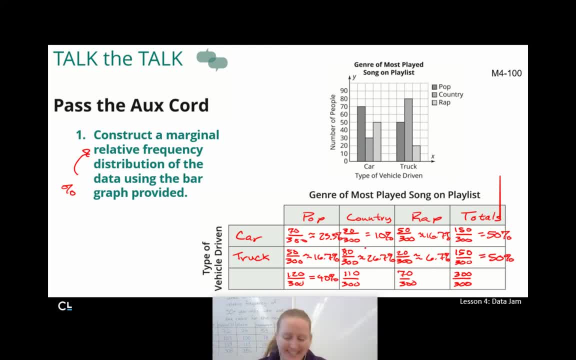 40%, That's nice. 110 out of 300. I did this earlier, I wrote it down- Is about 36.7% And, of course, 70 out of 300 is 23.3%, Except for some reason I can't write twos right now, Sorry. 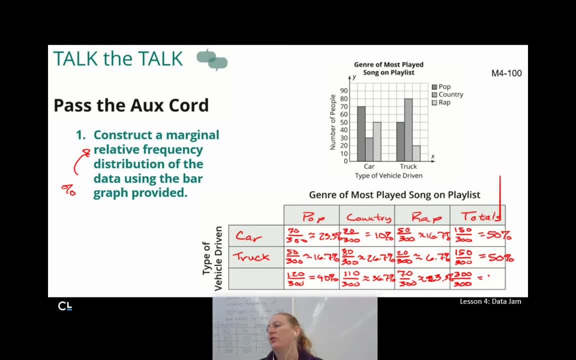 That's a 23. I'm sorry. And of course, 300 out of 300 is 100%. We knew that was going to be a thing Sweet. So now that we have our percents, you don't have to write a big old paragraph. 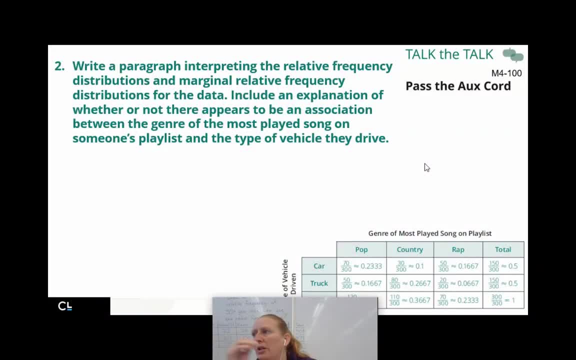 but can you just jot down some thoughts interpreting our relative frequency distributions or marginal relative frequency distributions, just comparing our percents, and include some kind of explanation about whether or not there appears to be an association between the genre of the most played song on someone's playlist and the type of vehicle they drive? Is there?